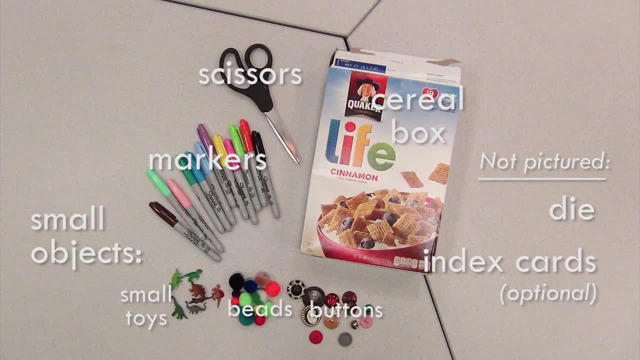 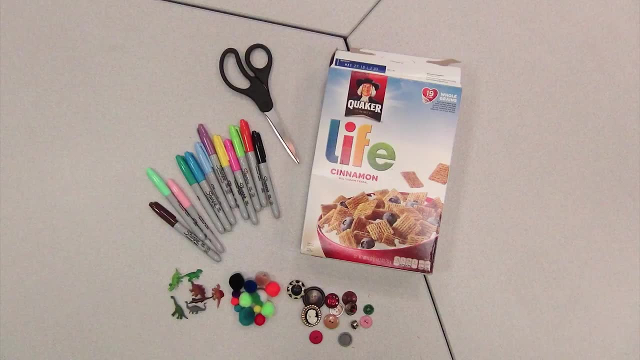 You can use buttons, beads or small toys. I borrowed these dinosaurs from a friend. Just make sure each piece looks different so you can tell them apart while playing. Now let's get crafting. First cut open the cereal box, then cut off the edges, Then cut off the edges. 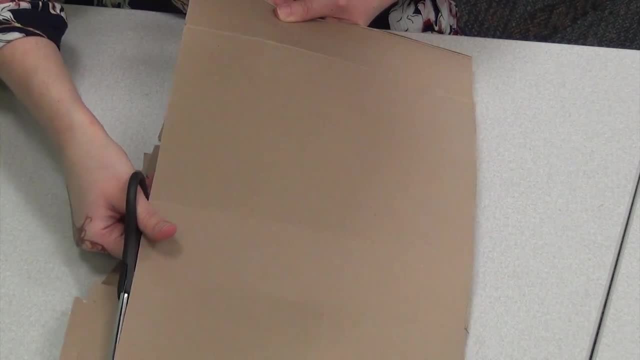 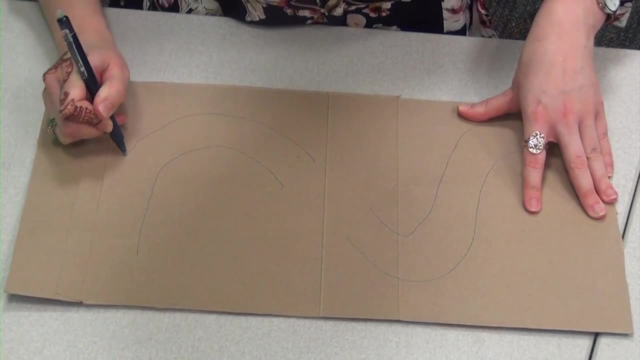 Cut off the top and bottom flaps, so you're left with a large cardboard rectangle. Bend the box back and forth at the creases to make it lay flat. Next, plan out your board game Sketch: a small twisty path with a start and a finish. 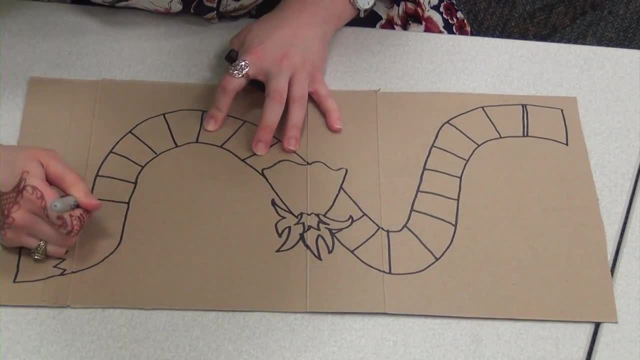 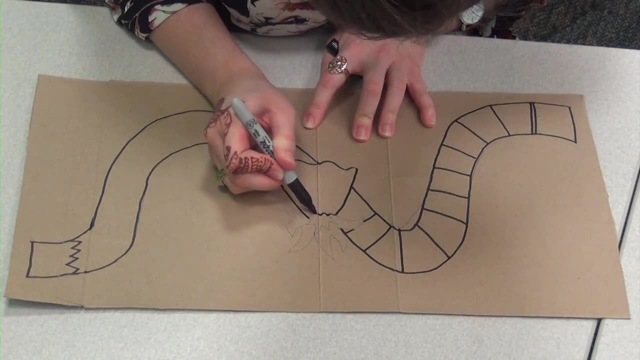 then add lines in the path to create spaces for players to move through. Think about what you'd like in the game. Do you want an obstacle in the middle or a story at the end? I added a volcano in the center. If a player lands on this, they'll have to go back to the beginning. 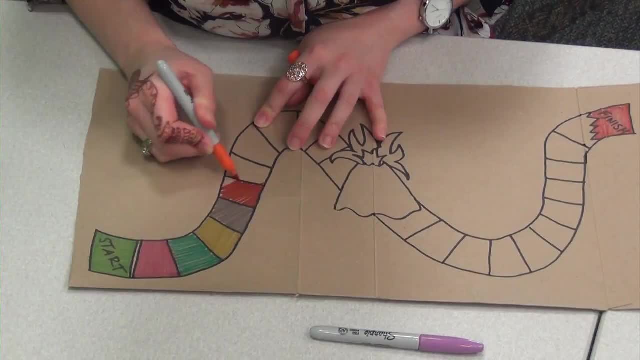 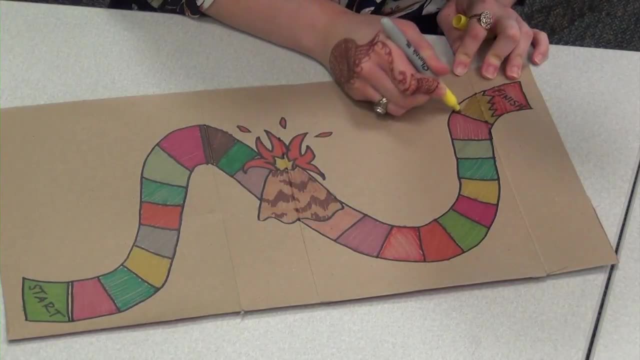 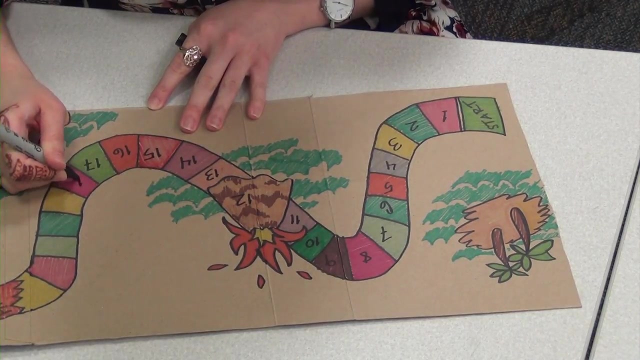 Now it's time to decorate your game. Invite your child to help you color the spaces. Your game has a theme like racing or oceans or whatever. Color your board to match. I added some jungle plants and islands to mine. Finally, number all the spaces in the game and find small objects to use as game pieces. 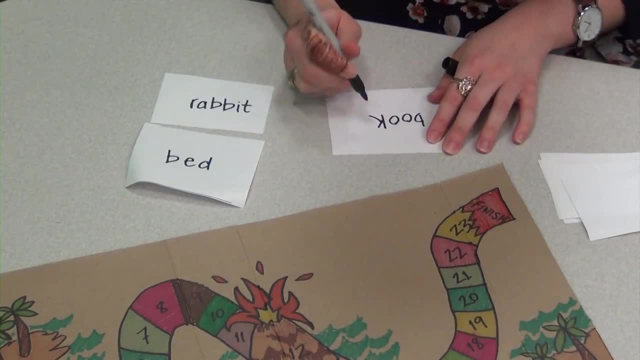 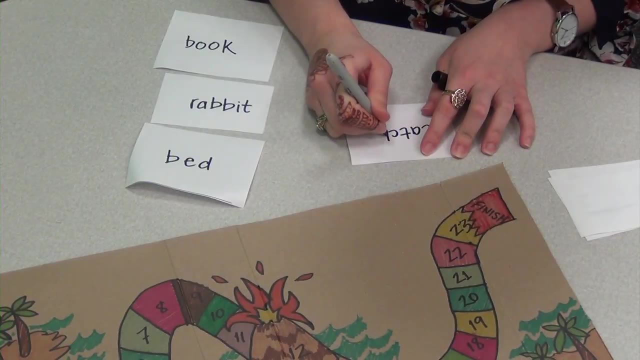 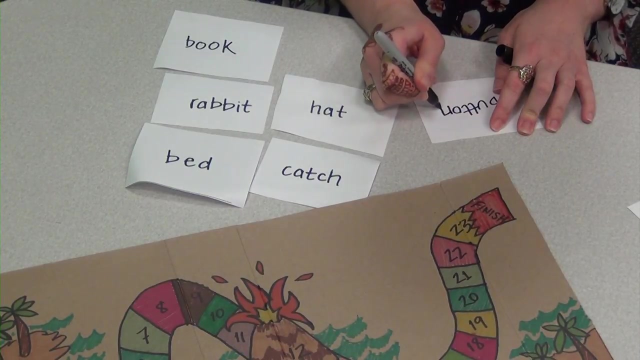 One more step. This is optional To make the game challenging for older children. take index cards and write different small challenges on them. It could be sight words to read or spell, small math problems to solve and more. If you have an age-appropriate trivia deck for your child, this would be a great way to use it. 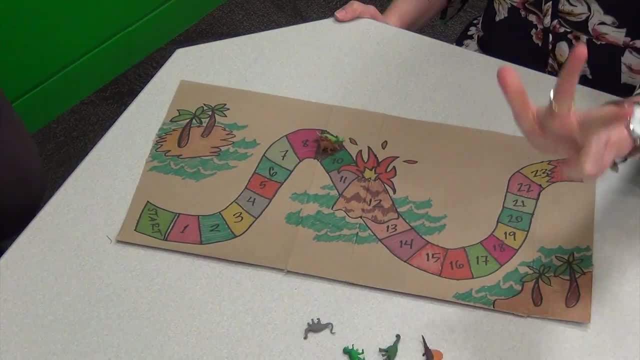 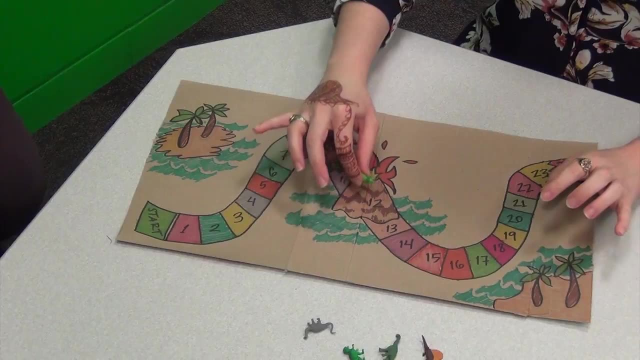 Now you're ready to play. Each player rolls the die and moves the number of spaces they rolled. This is where the counting practice comes in. Oh no, That's the volcano. Back to the beginning. For older children, have them draw a card and answer the question or challenge on it. 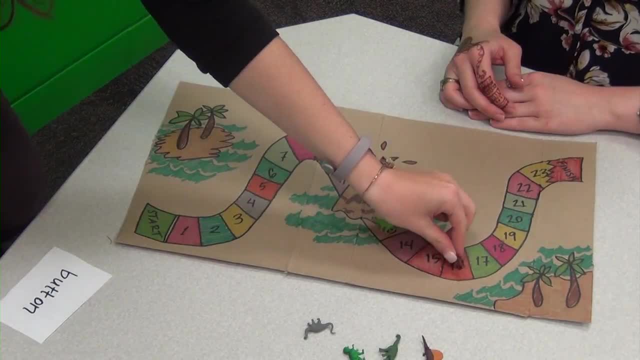 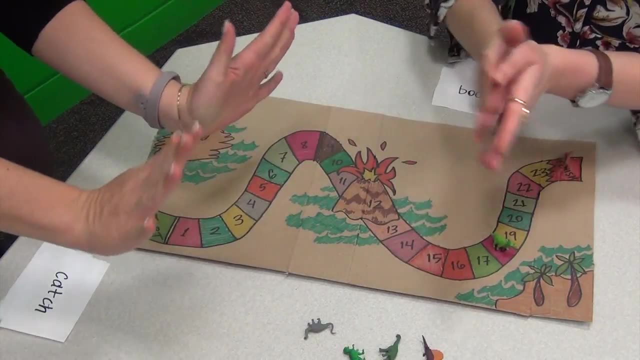 If they answer correctly, they can roll the die and move forward. If not, they can stay put and wait until their next turn. And, of course, whoever reaches the end first wins the game. Enjoy this fun game together. Consider adding little prizes to make game night more fun. 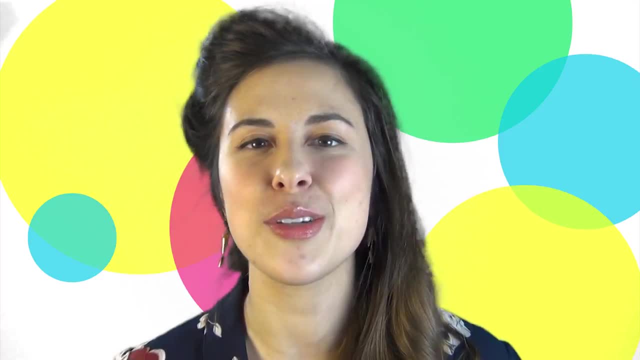 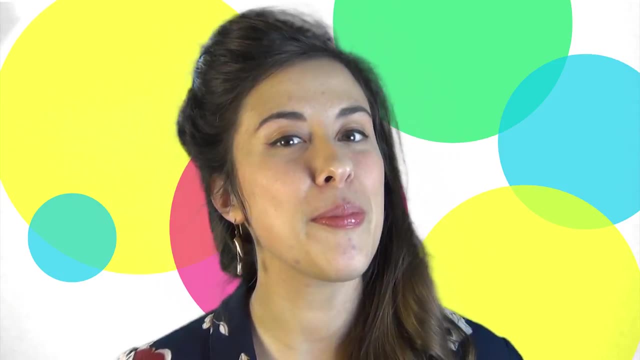 An extra piece of dessert, a funky pencil or a personalized drawing from mommy or daddy. Don't forget to end game night with our favorite activity: reading a book together. Happy playing and happy making Subtitles by the Amaraorg community.